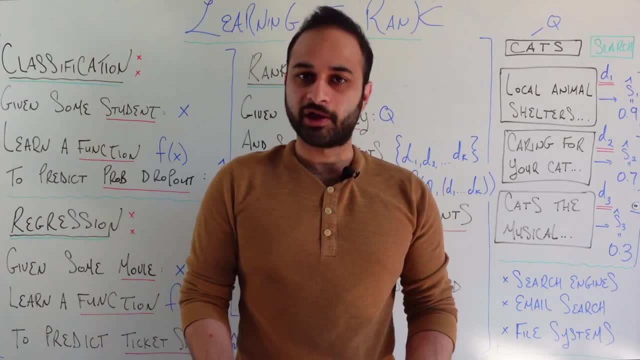 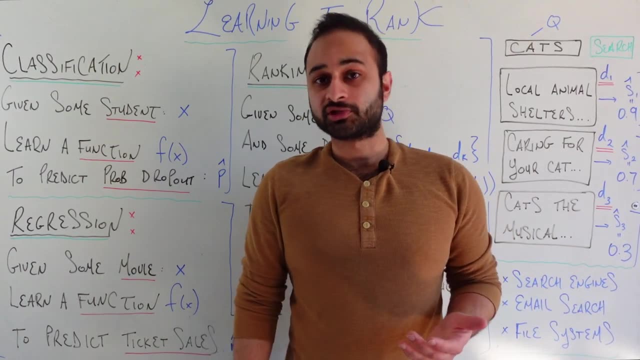 likely to drop out. maybe we send some resources, help them out in some way. So that is a typical classification problem. We also have regression problems and we've talked a lot about how to solve those. For example, given some movie x, so x is just some kind of feature vector about a movie. 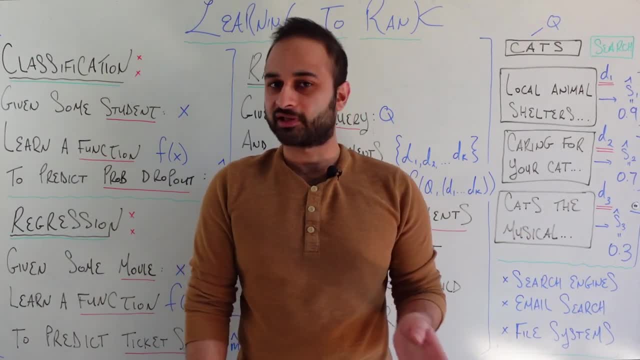 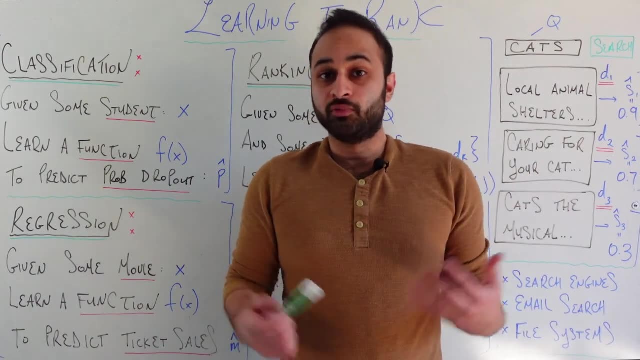 like which actors are in, how much do they spend on the movie, stuff like that. Can we learn a function f of x which is going to predict the ticket sales? m hat m just for money that the movie will make? So this is trying to predict some kind of continuous value. 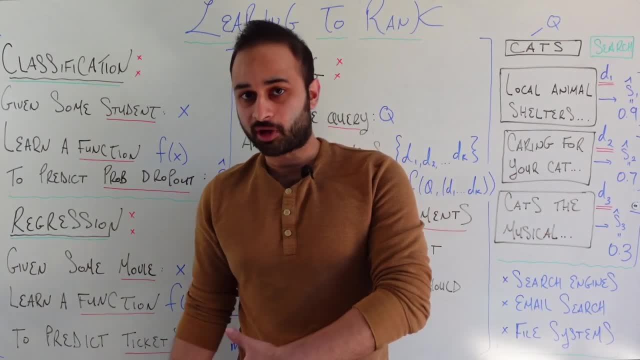 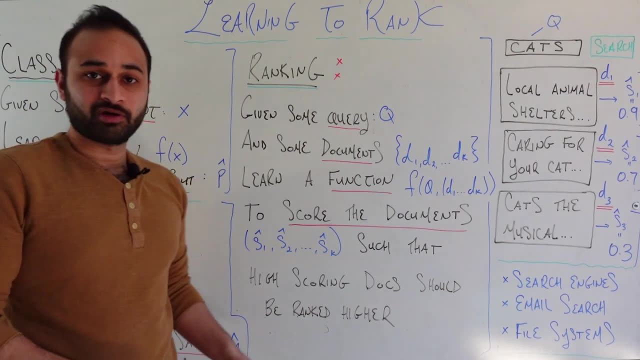 instead of some kind of discrete value, and so we call these regression problems. Now, here comes the new class of problems. What I'm going to do first is walk out here and I'm going to describe the setup of this problem, and then I'll talk about it in a more human, understandable way. So we 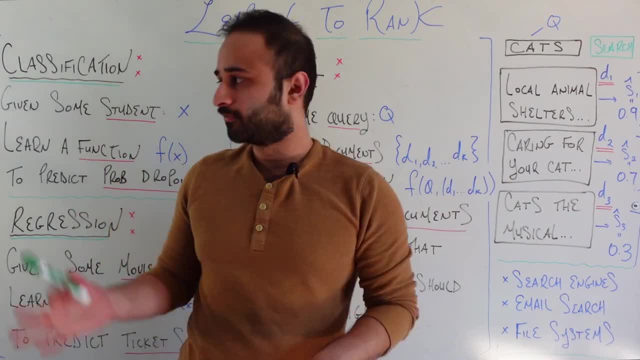 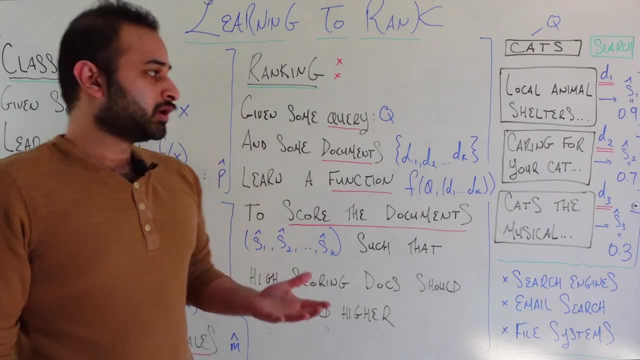 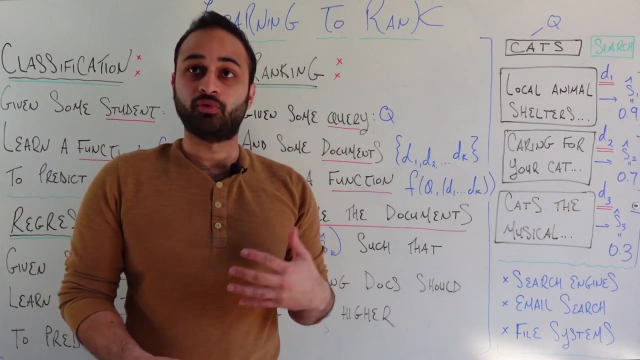 understand exactly what it is we're trying to solve and how. it's fundamentally different from these guys. So this class of problem is called ranking problems or starting to rank. So officially, given some kind of query queue, I'm choosing to use this nomenclature of queries and documents just because, if you do any research in this field or read, 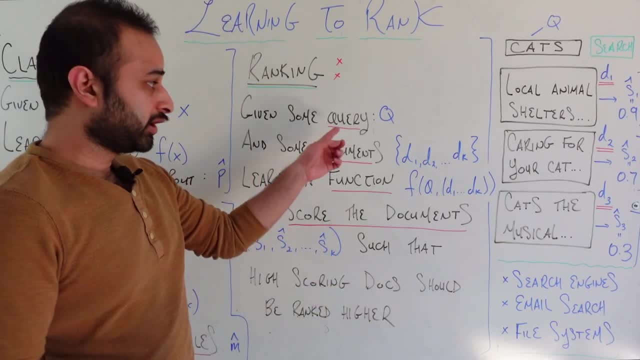 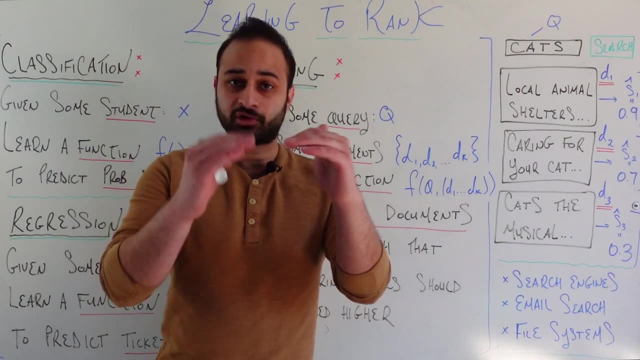 papers. that's a lot of times what you'll see. But you can think of as a query, just as any kind of search you might put into a search engine, for example, And you can think of documents as the results that are returned by that search engine. So, given some kind of query queue and some 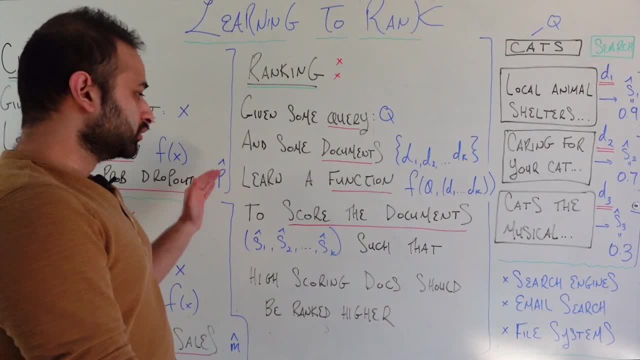 documents d1 through dk. you want to learn a function f of x which is going to predict the ticket sales m hat. So this class of problems is going to have a function f, a function of that query and those documents which is going to be able to. 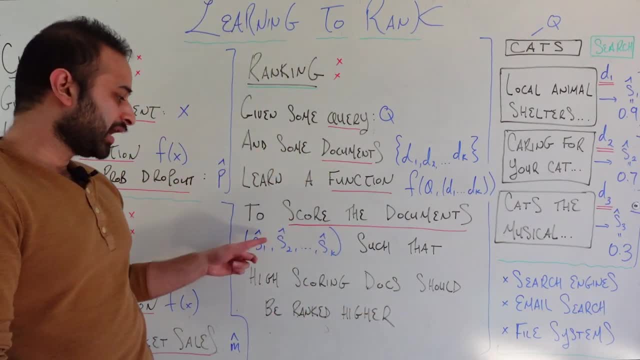 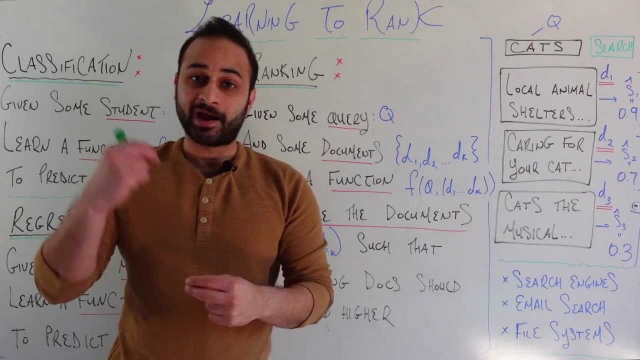 output a score for each document. So it's going to give you s1 hat, s2 hat all the way to sk hat, such that the higher scoring documents should be ranked higher for that particular query queue. Now that I've basically read what's exactly on the board, let me talk about it in a more. 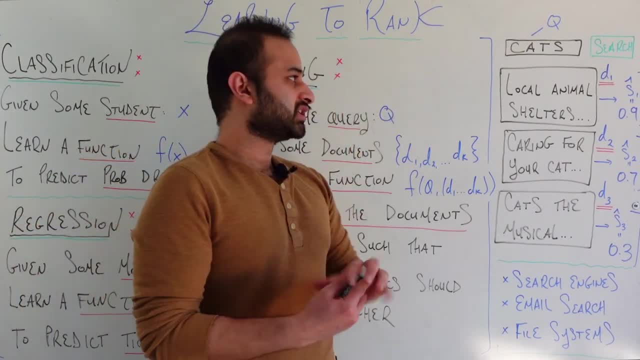 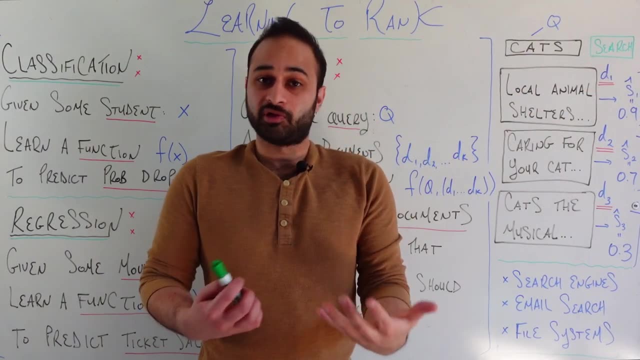 human, understandable way. So, for example, let's say you're designing the world's first search engine for animal lovers And let's say someone types in the query cats. So this can be thought of just as a search or a question you might have. So they're going to. 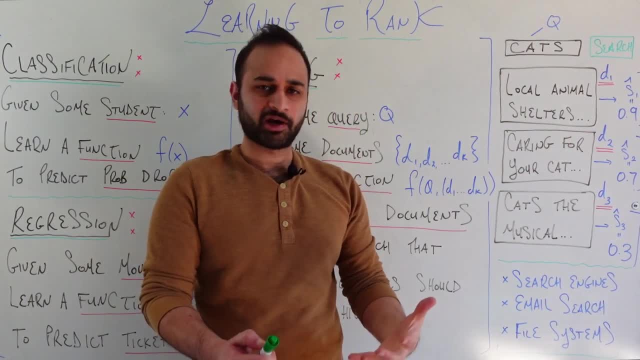 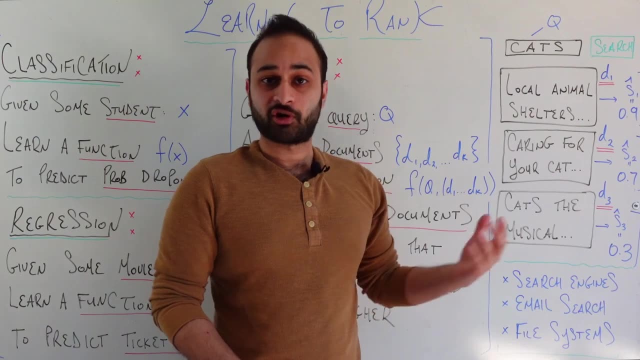 type in cats and hit the search button And, as you might expect, we're going to get a populated list of documents or results that are going to match their query. For example, the first one's on local animal shelters, the next one's on caring for your cat and the last one is about cats, the musical. 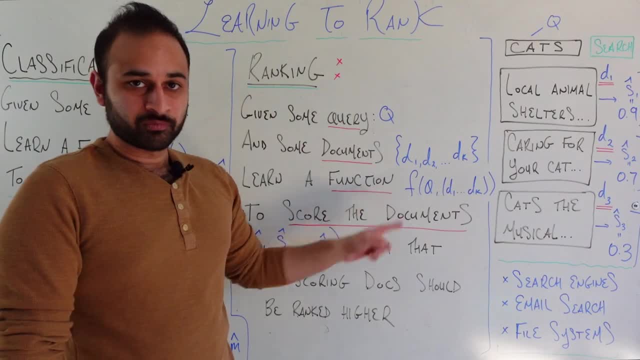 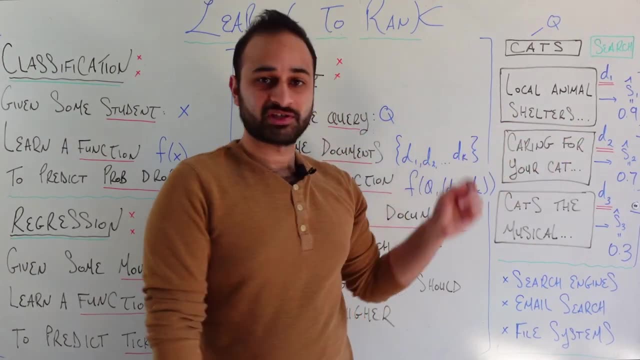 Now this function that we learned is going to output a score for each of these guys. For example, let's say the score for this one, And then we're going to output a score for each of these guys. So the first one is 0.9, the score for this one is 0.7, and the last one is 0.3.. And that is exactly. 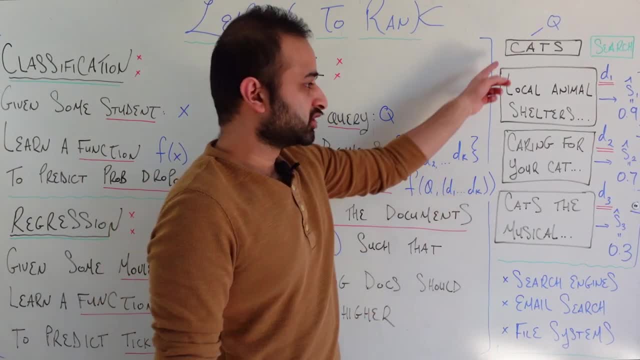 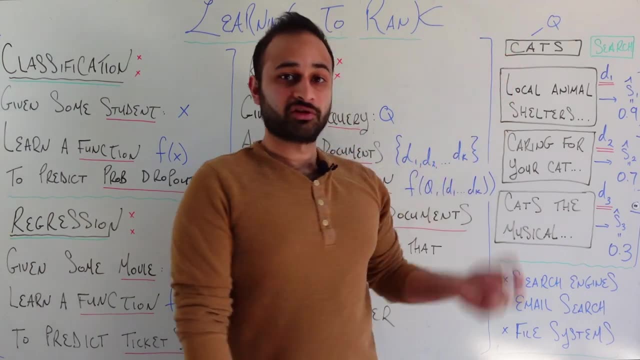 the score we use to rank the documents for this particular query, because we believe that the scores that are higher align with documents that are more relevant to the query the user typed in. So at the heart of this ranking, of this learning to rank problem, is: 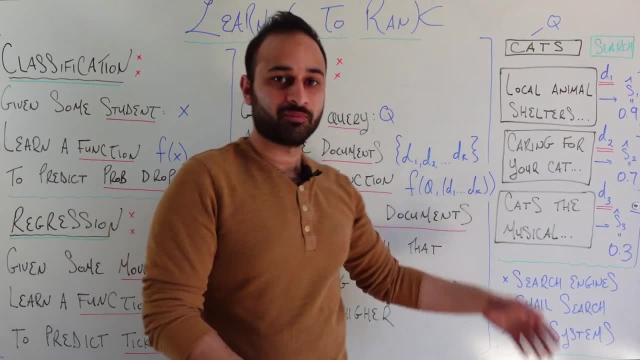 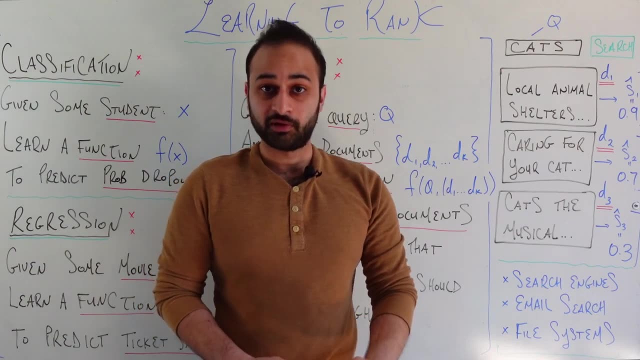 exactly the fact that these scores are what are used to rank the documents in relevance order for the user, based on what search they type in. And now I think it's very important to understand how this is fundamentally different from a classification or a regression problem. 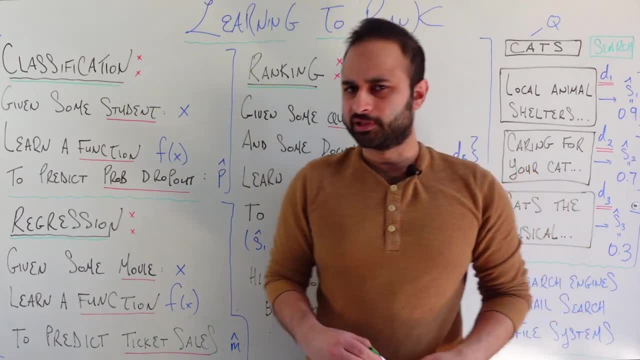 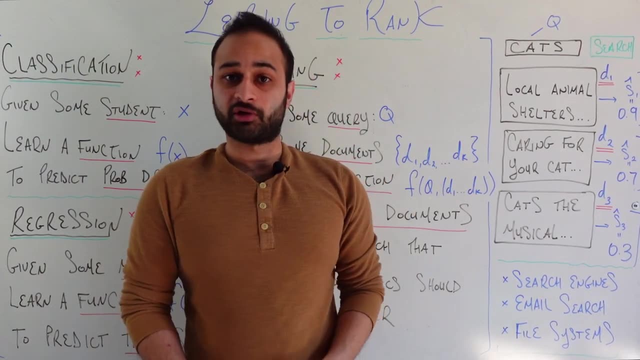 In a classification problem we are doing some kind of predicted probability. So you might think this is classification, because can't we just predict whether or not some kind of document is relevant for a particular search? That could be a crude way to do it. 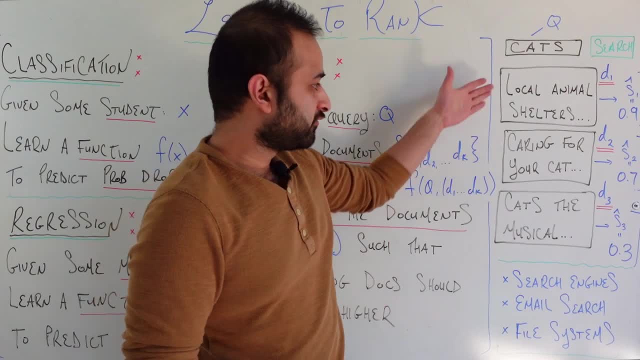 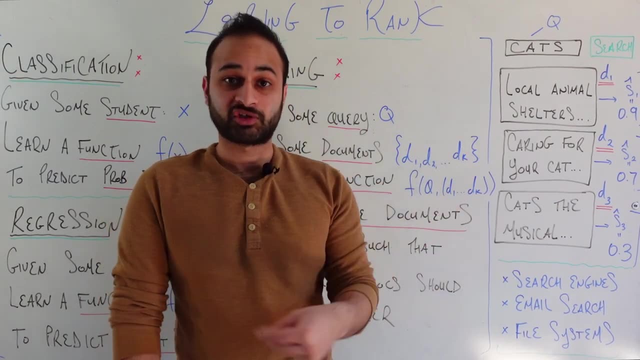 but you'd be leaving a lot of information on the table because these documents are fundamentally related to each other. We're not considering each one independently because they're all related through the fact that they are possible documents for a given query. So we're not considering each one independently because they're all related through the fact that they are possible documents for a given query. 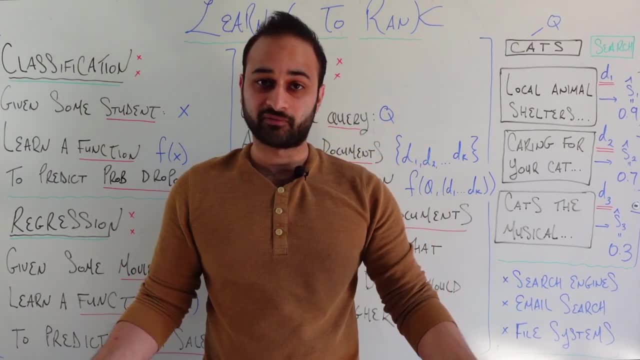 So we're not considering each one independently, because they're all related through the fact that they are possible documents for a given search. If you had a different search, like dogs, you would have a different set of documents. So it really is this kind of grouped problem where you have a query and a set of possible. 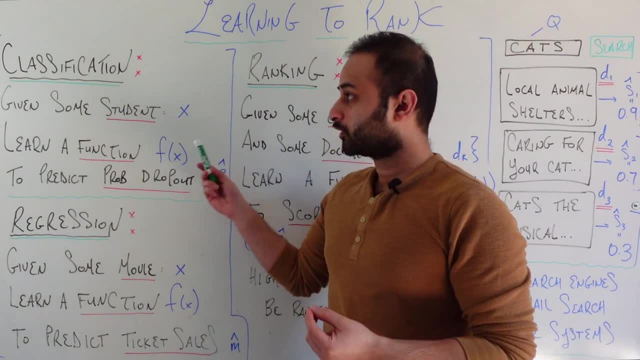 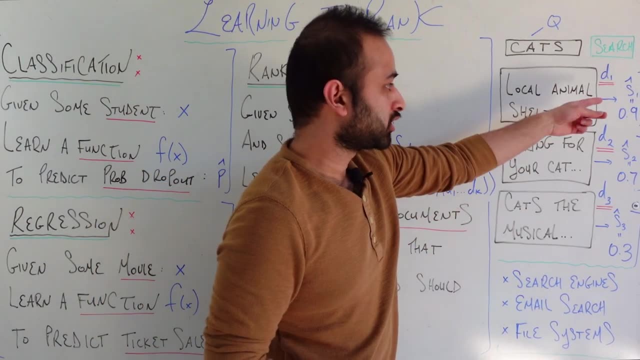 documents and they need to interact with each other in a way that a typical classification framework can't really do. You might think this is a regression problem, because can't we just use the regression techniques to find these scores? Well, again, that could be a. 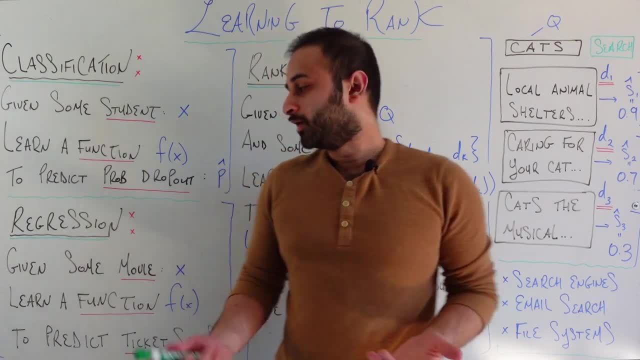 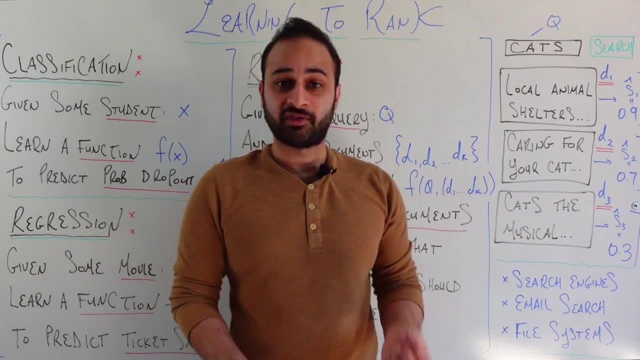 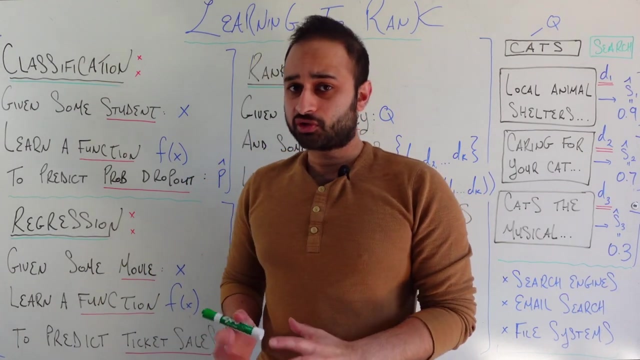 crude way to do it. but again we're doing the exact same problem where a regression framework doesn't really think about the interactions between observations in the dataset, whereas here we do explicitly need to think about those interactions. Which one should be ranked higher than the other? So for that reason this is neither a classification or a regression.